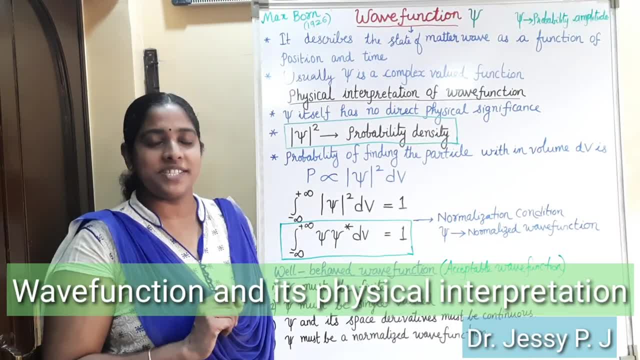 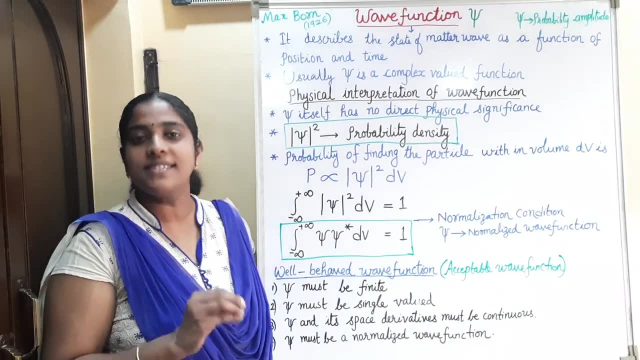 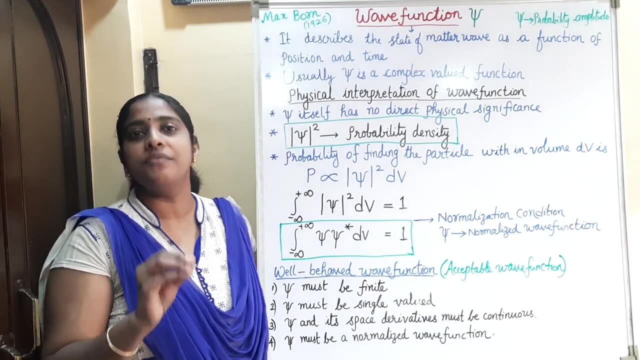 Hi all. today we can discuss about wave function As, per de Broglie hypothesis, a moving particle is associated with a matter wave, that is de Broglie wave. We know that every wave is described by some wave variable that varies with the space and time, For example, in the case of water waves. 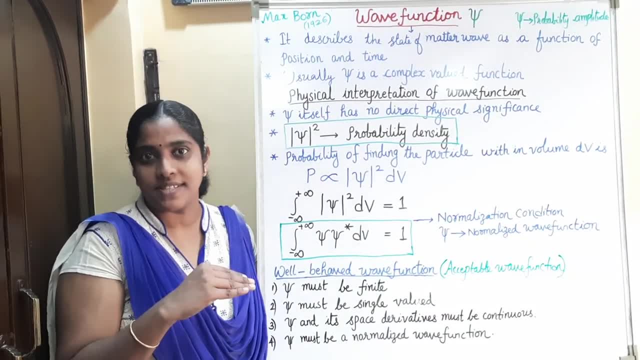 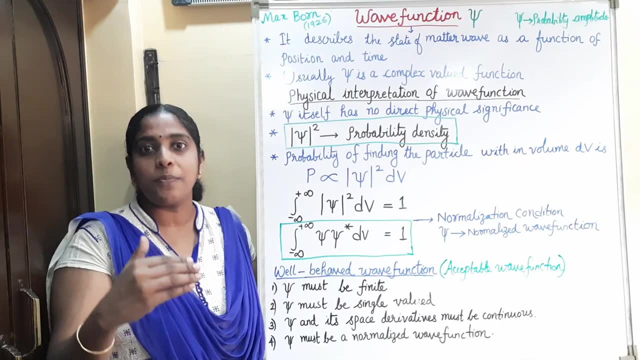 it is the height of the water from the surface that varies. In the case of sound, it is the pressure. that is, when sound wave propagates, the pressure variation that is propagating as compressions and refractions In the case of light wave, the electric field and magnetic. 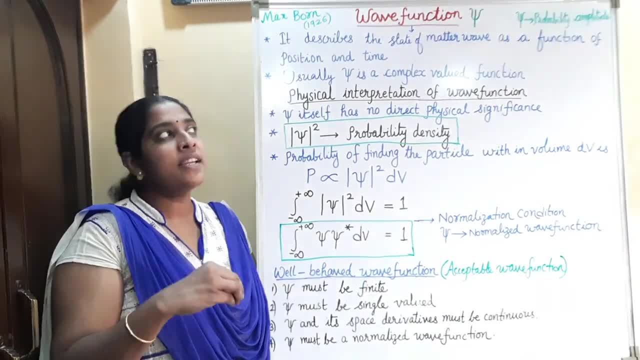 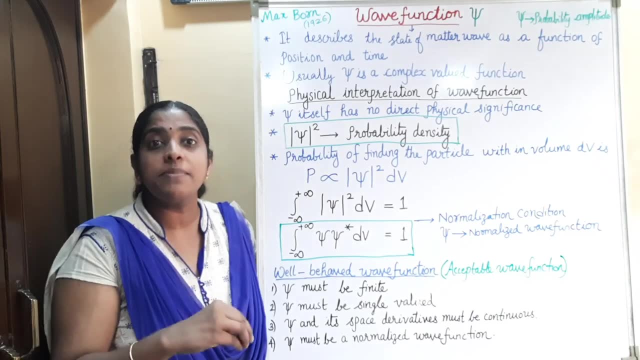 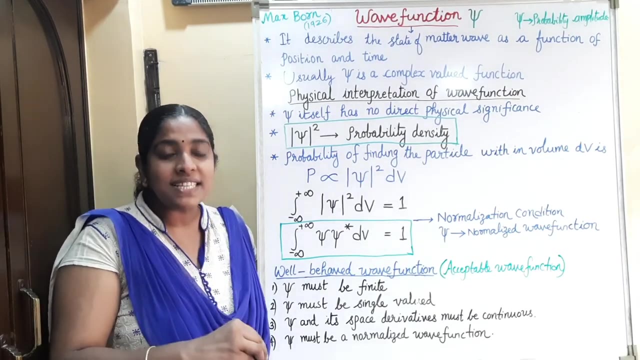 field describes the behavior of that radiation. Then, in the case of de Broglie wave, that is matter wave, what will vary? What describes the behavior of de Broglie wave in space and time? Then that quantity that describes the state of 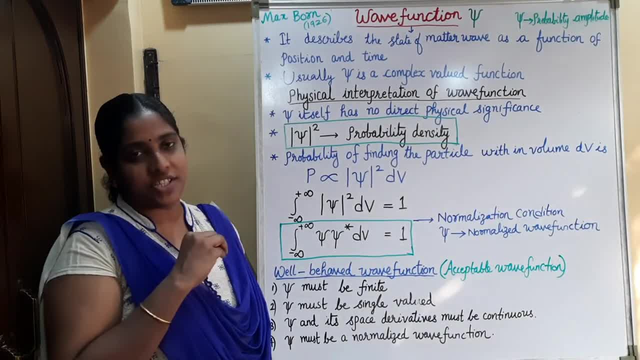 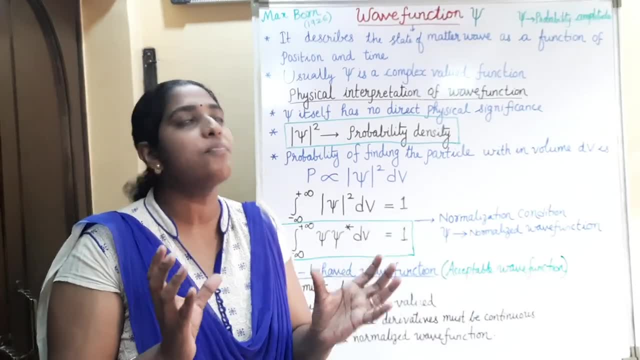 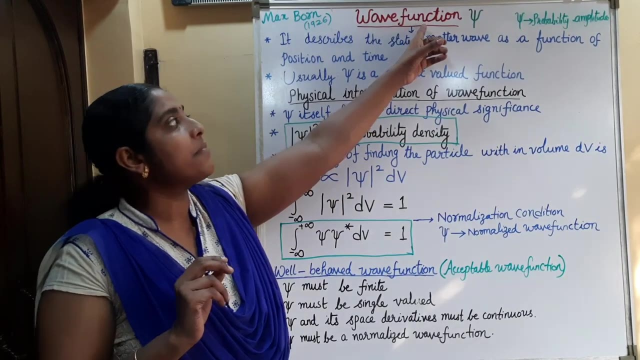 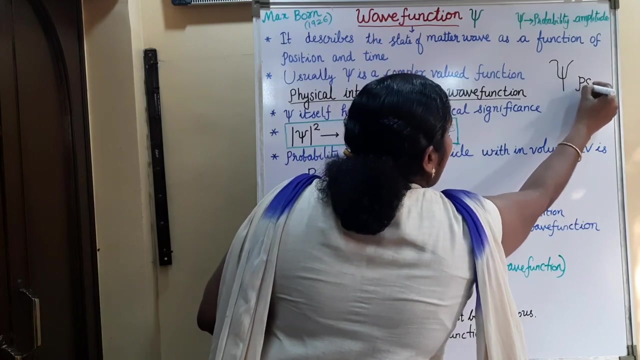 the matter wave that is known as the wave function. So the wave function is a quantity that describes the behavior of matter wave as a function of position and time. This wave function is denoted by a threshold-like symbol. This symbol is a Greek letter. It is read as psi. 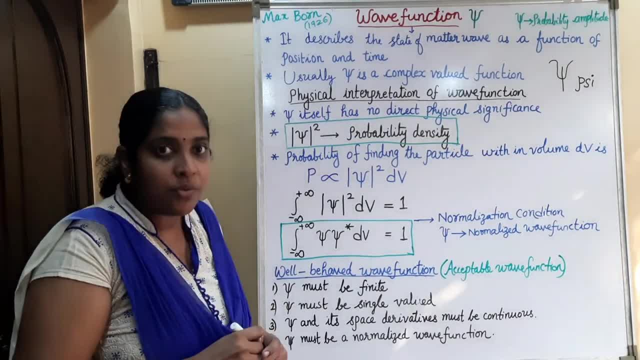 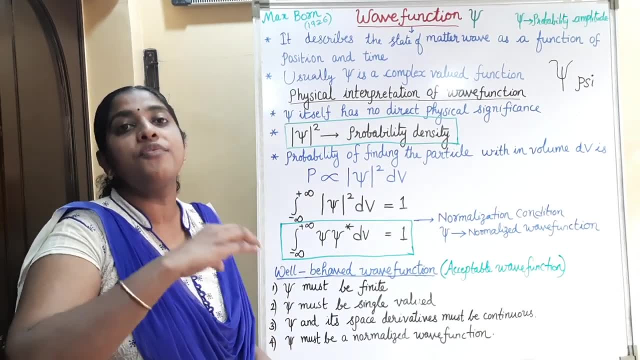 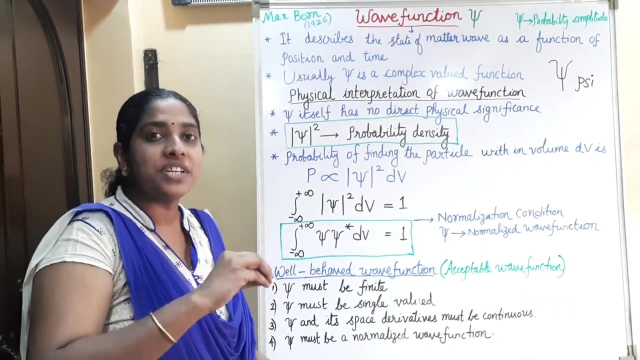 P is silent, psi. So the wave variable that varies in space and time, which describes the state of de Broglie wave, is known as the wave function. So the variation in the wave function that makes up the matter wave. 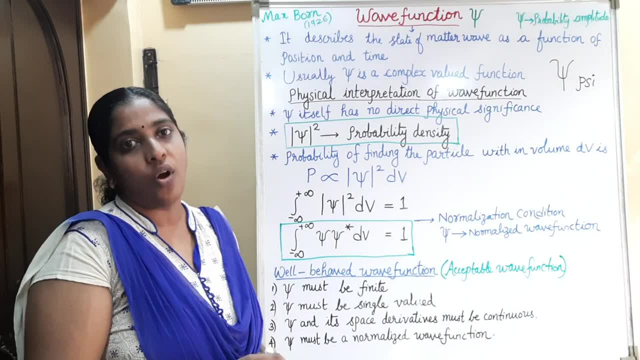 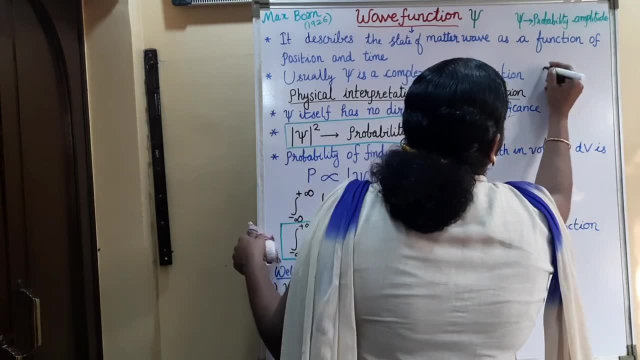 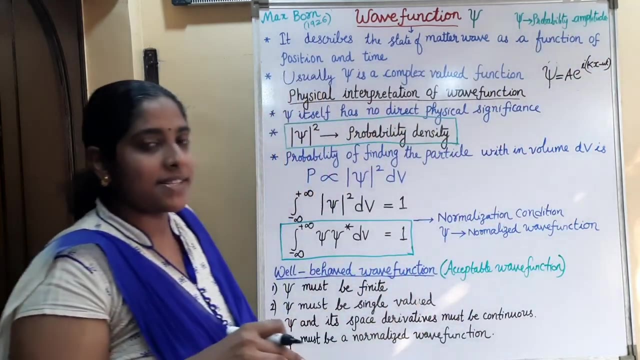 So generally the wave function psi is a complex valued function. For example, we can write this psi as a e raised to ikx minus omega t, So this i makes it complex. So generally this wave function is a complex valued function. 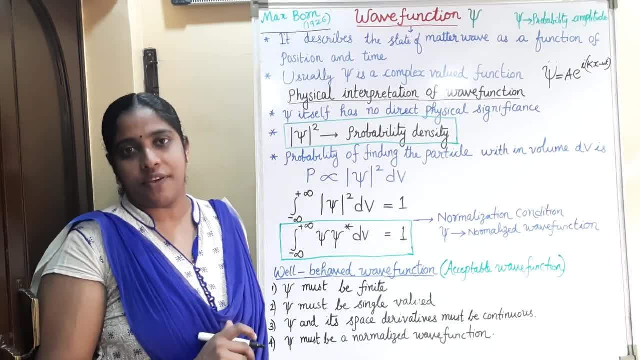 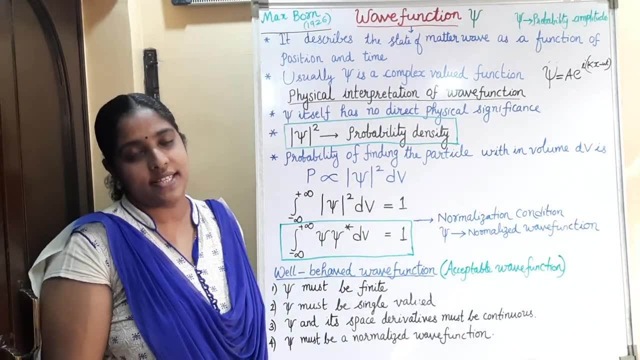 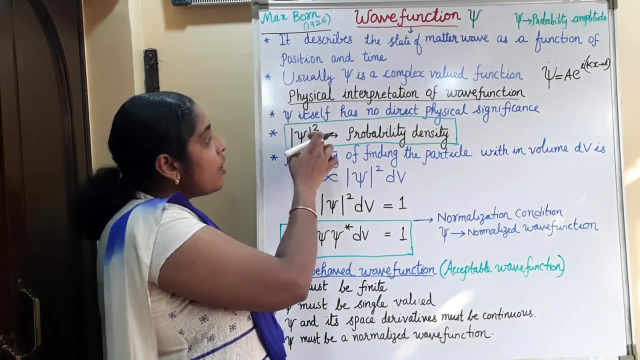 Now we can see what is the physical significance of this wave function. The interpretation of this wave function was given by the scientist Max Born in 1926.. This wave function, psi, itself has no physical significance, But the square of the absolute value of this wave function. 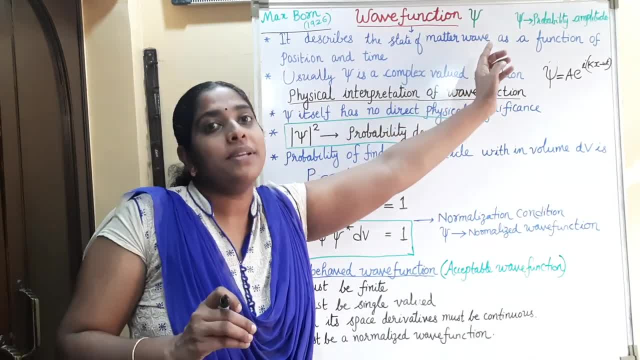 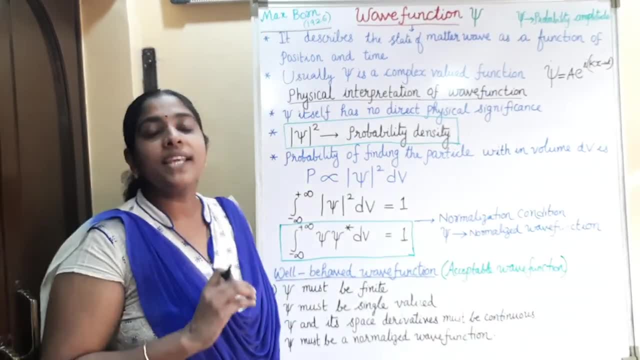 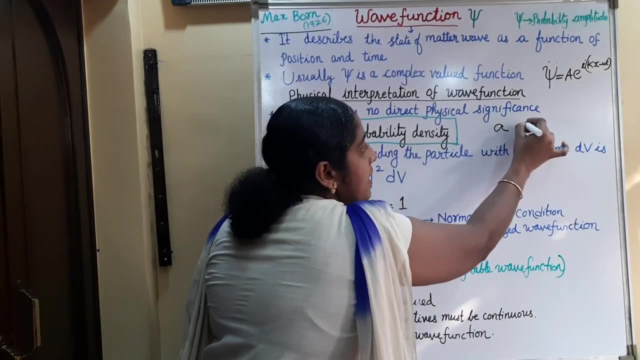 gives the probability density. If psi is the probability amplitude, the square of the absolute value of the wave function gives the probability density. We can compare this with the case of light, that radiation, That is. if a is the amplitude of the light, what is the intensity? 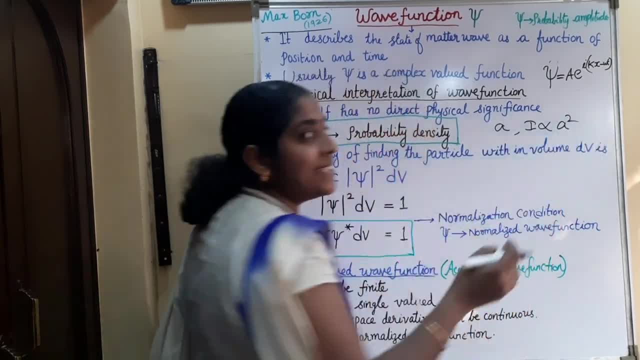 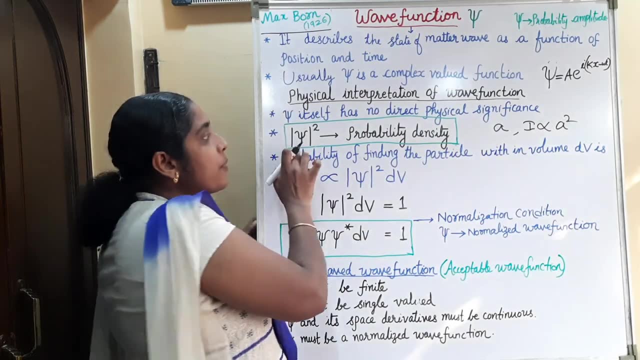 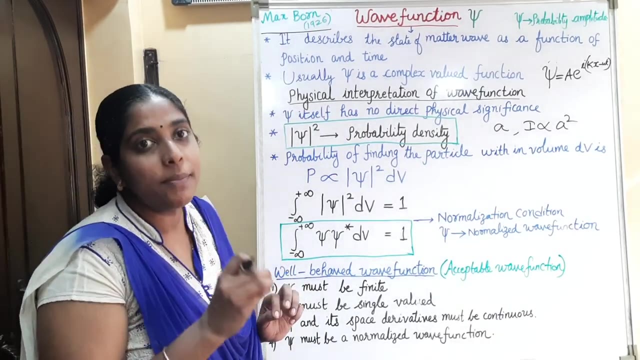 that is proportional to the square of the amplitude and that is the photon density, that is the number of photons in unit volume. Similarly, the psi is the probability amplitude, Then the square of this wave function. that gives the probability density. What is probability? 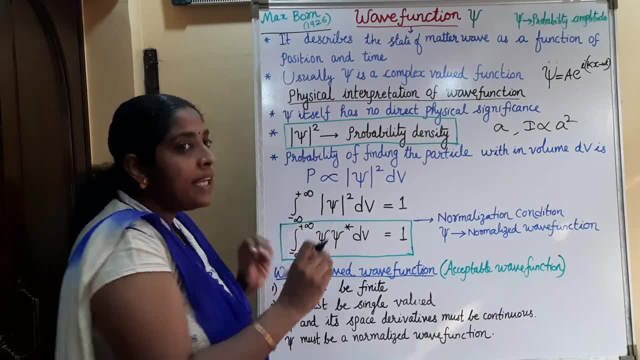 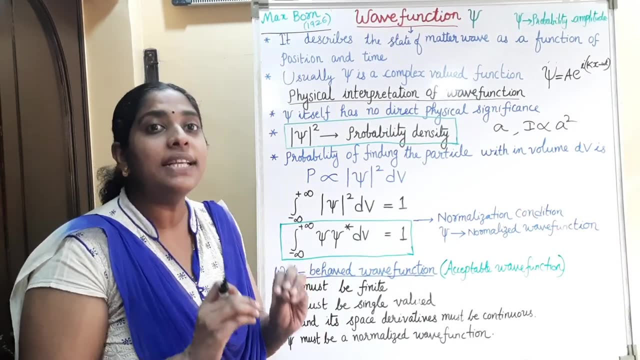 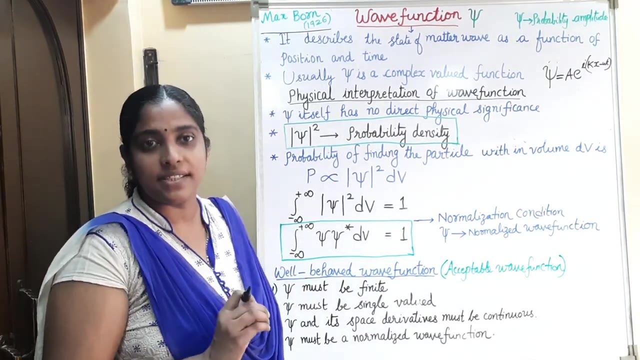 density. Probability density is the probability of finding the particle in that region. What is the probability density in a region? It is the probability of finding the particle in that region. Why? psi itself has no physical significance directly, Because if you are finding the probability of something in a region, that value is equal to the probability. 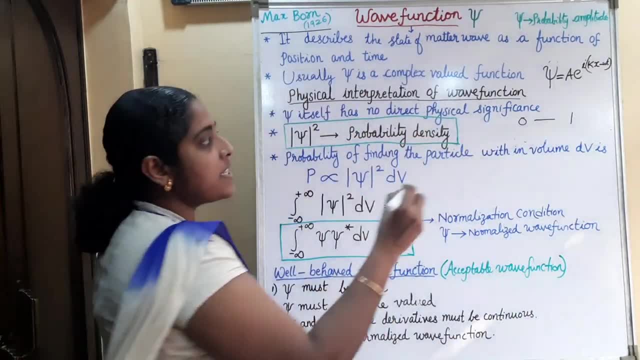 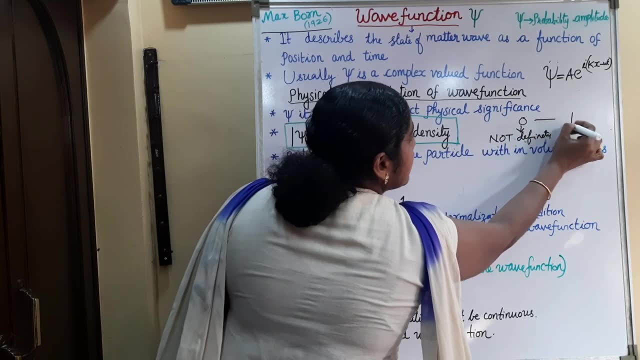 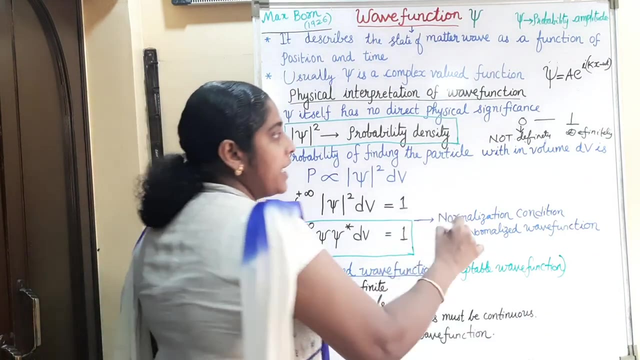 that lies between 0 and 1.. What is the meaning of 0?? That means that something is not definitely there. Then what is the meaning of 1? That is, the particle is definitely there, That something is definitely there. That is 100% probability In between, if we are considering 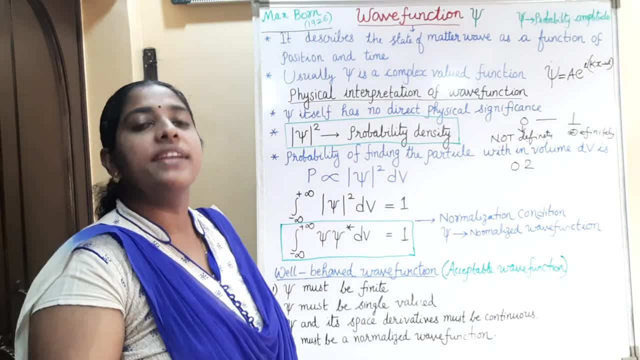 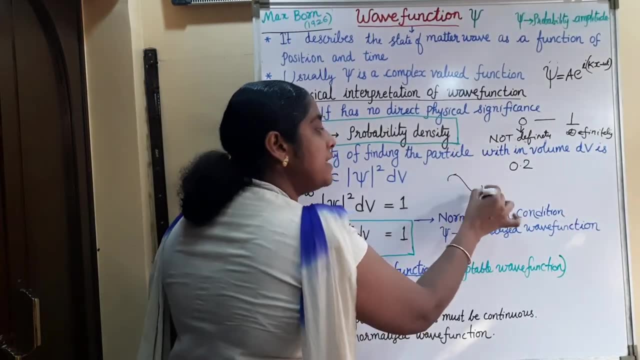 0.2,. that means 20% of chance of finding something in that region. Now, in the case of wave, the amplitude can be positive and negative. in some regions The wave function cannot be seen by any of these regions. We have to know that in a region the amplitude cannot. 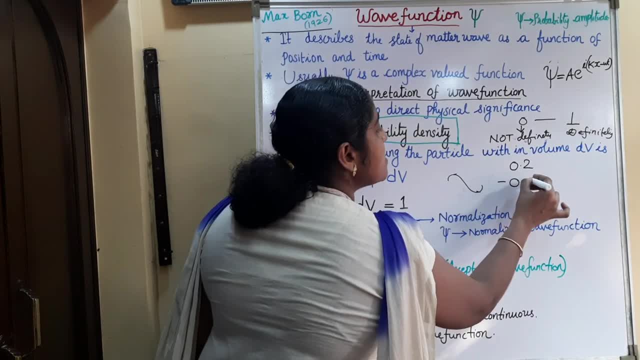 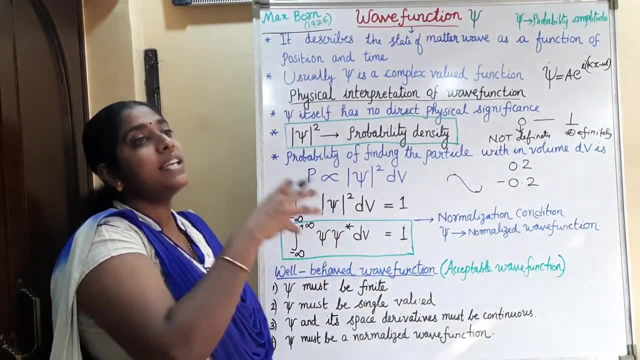 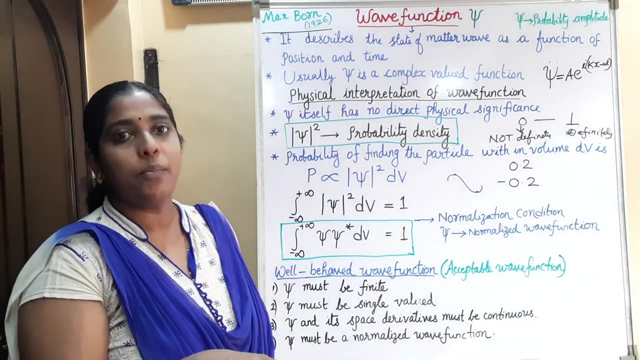 so if you are saying the probability as minus 0.2, it is meaningless. so that's why we are taking the probability density as the square of the wave function. so when we are taking the square, what happens, we will get a real positive quantity. so the probability density is given by the square. 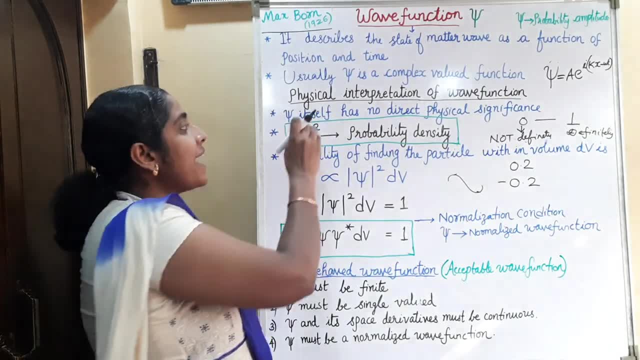 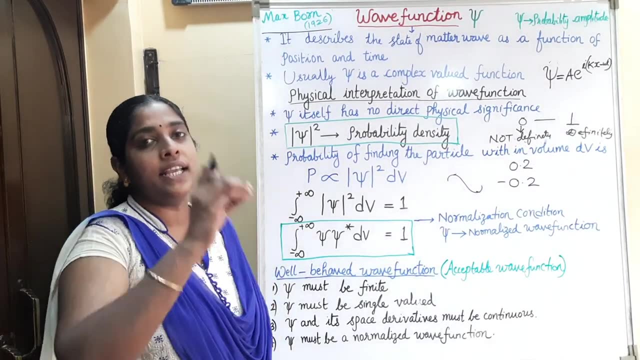 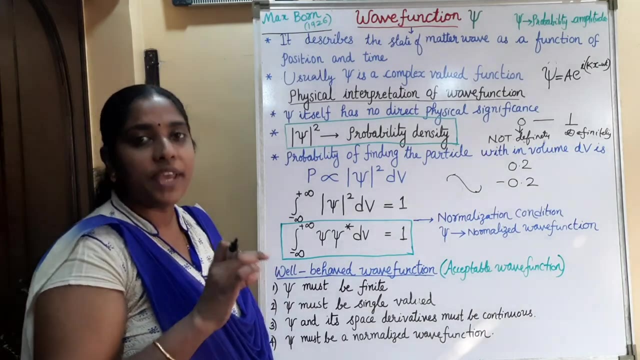 of the absolute value of the wave function. so psi itself has no direct physical significance. so we can say that the probability of finding the particle in a volume d v that is proportional to the square of the modulus of wave function in that region, that is, p, is proportional to psi square d v. 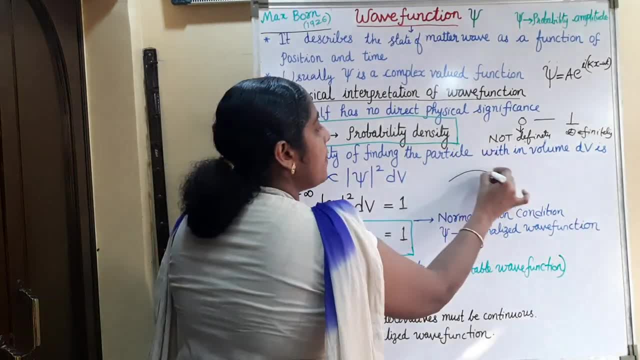 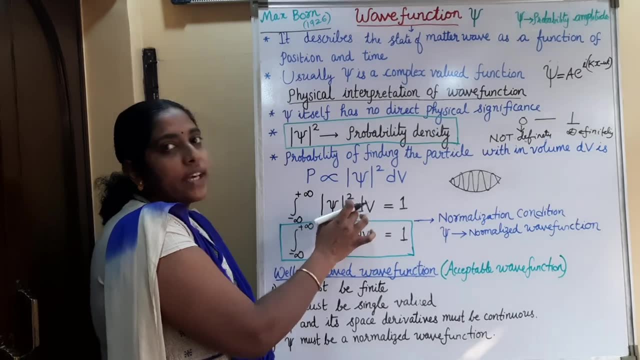 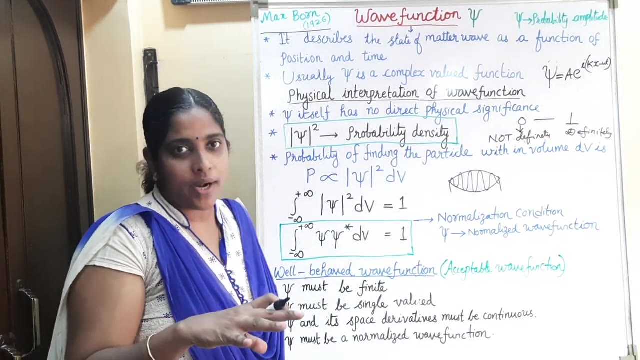 now, if you are considering the wave packet, the probability of finding the particle inside the wave packet is is equal to psi square dv. so if you are taking from this point to this point, the probability of finding that particle will be equal to one, because the particle is somewhere within the 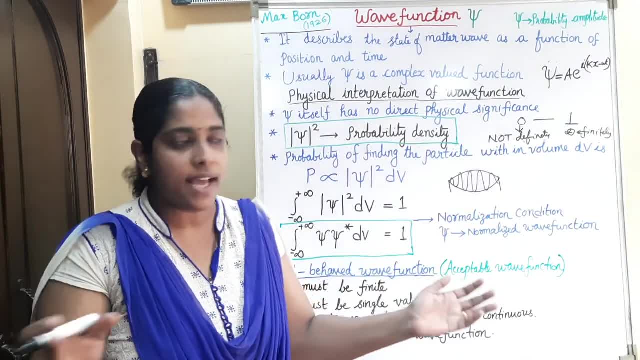 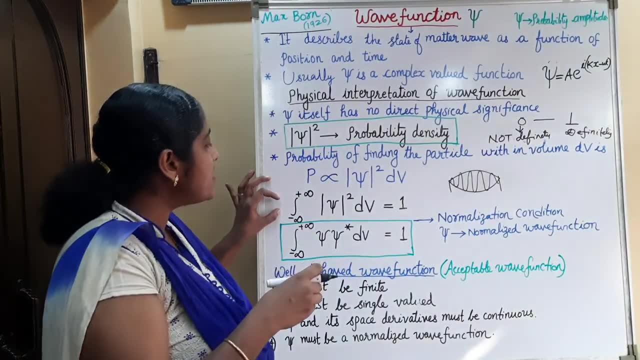 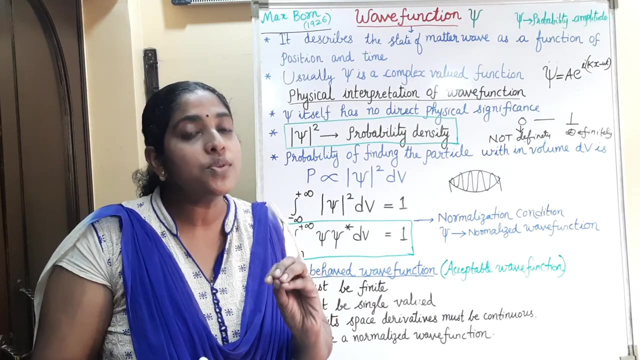 wave packet. so if you are considering the ender space, that is, from minus infinity to plus infinity, the particle will be somewhere there. so we can say that minus infinity to plus infinity, psi square dv is equal to one. remember this wave function used to describe the behavior of a single. 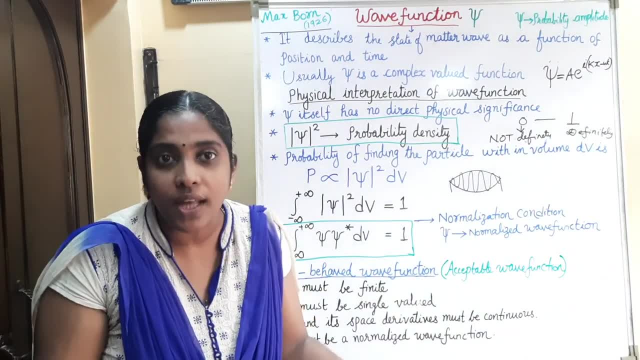 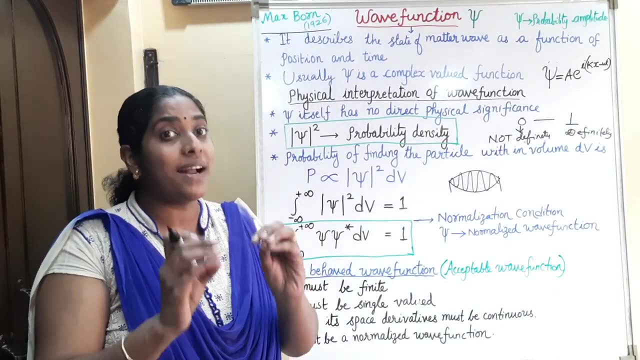 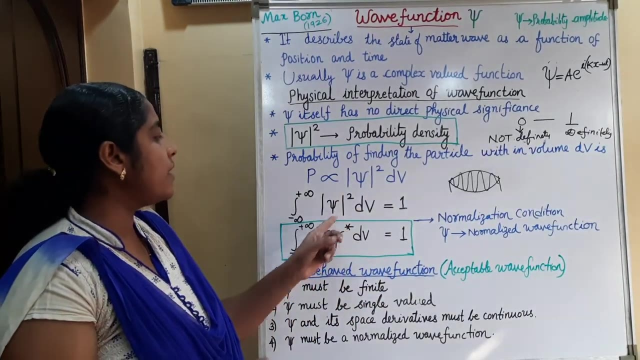 particle, not the statistical distribution of a number of any such thing. so the minus infinity to plus infinity, psi square dv is the probability of finding the particle in the ender space that will be equal to one. so we can also write this psi square as psi, psi star. minus infinity to plus. 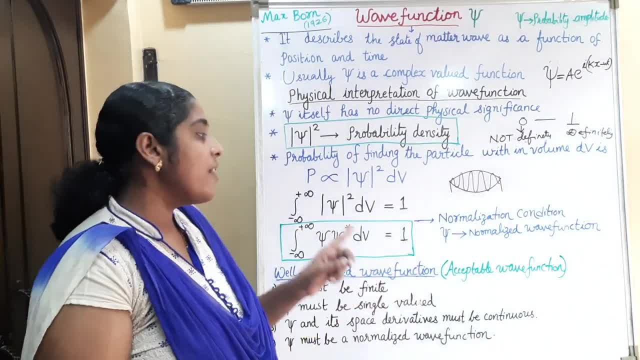 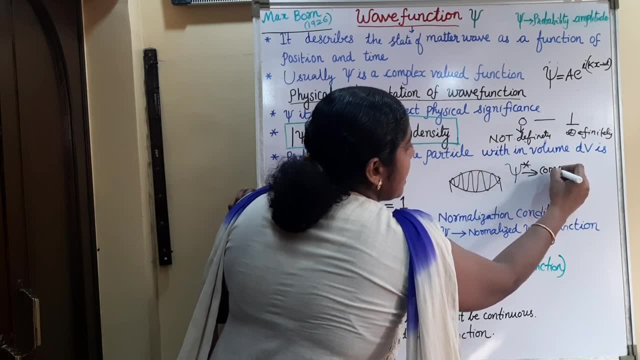 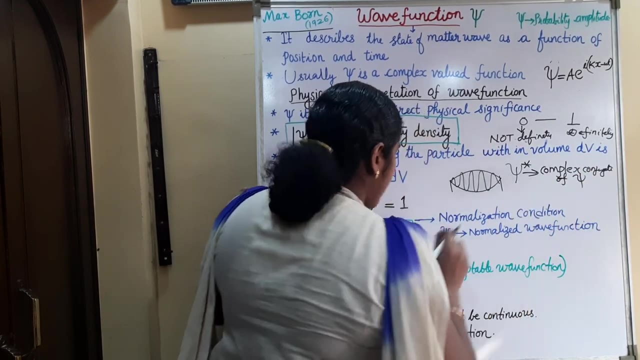 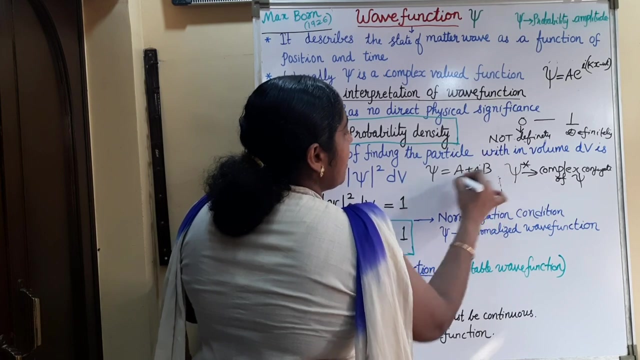 infinity. psi, psi star, dv equal to one. what is this psi star? psi star is the complex conjugate of this psi. what is psi star? psi star is the complex conjugate of psi. for example, if you are taking psi as a plus ib, okay, psi is equal to a plus ib. then to find the complex conjugate, just replace this i by minus i. 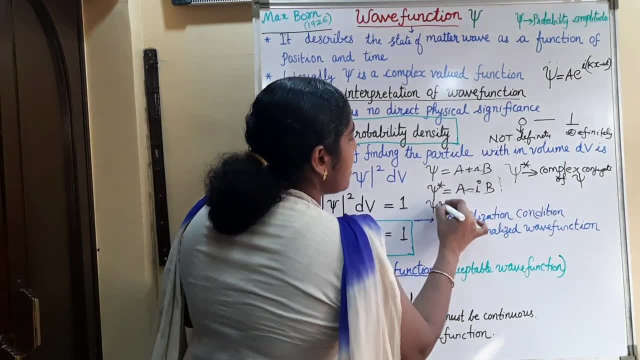 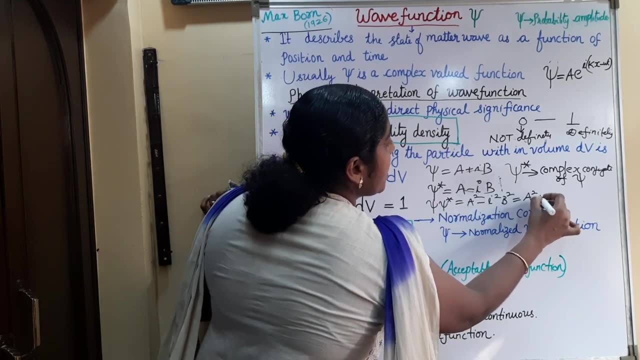 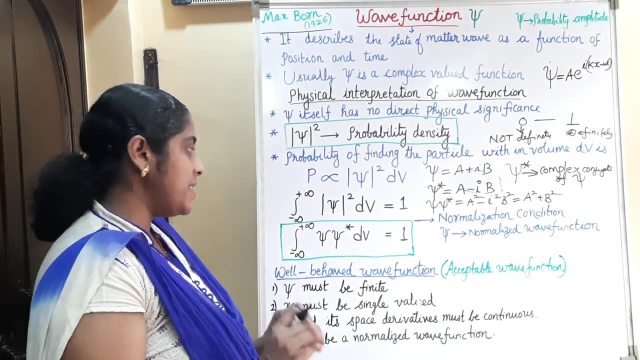 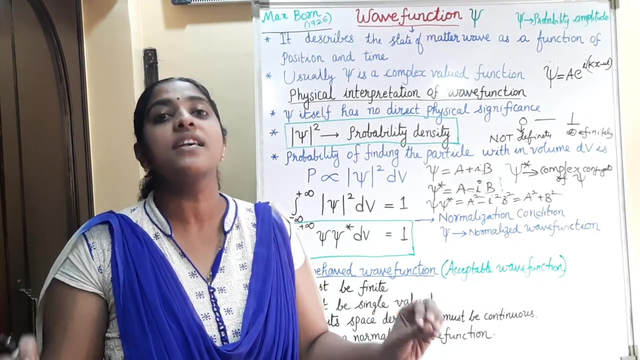 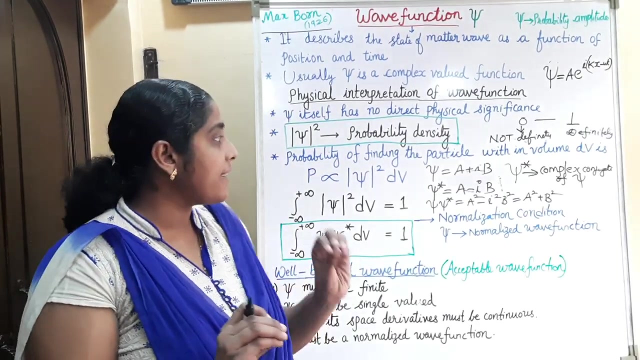 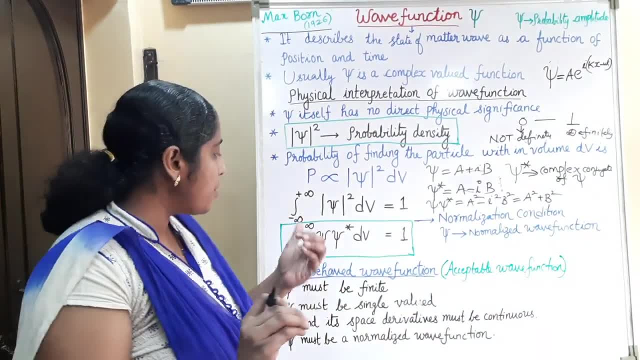 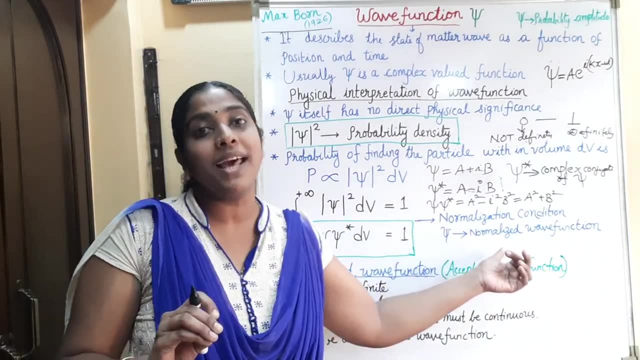 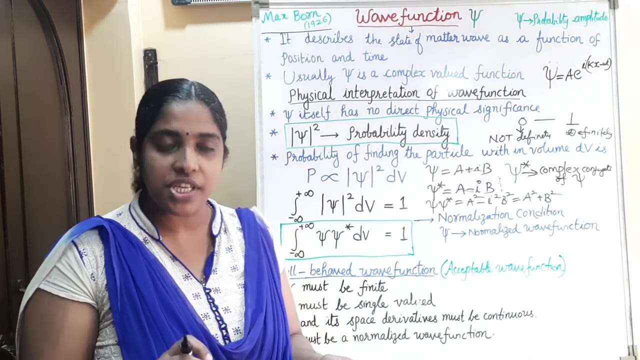 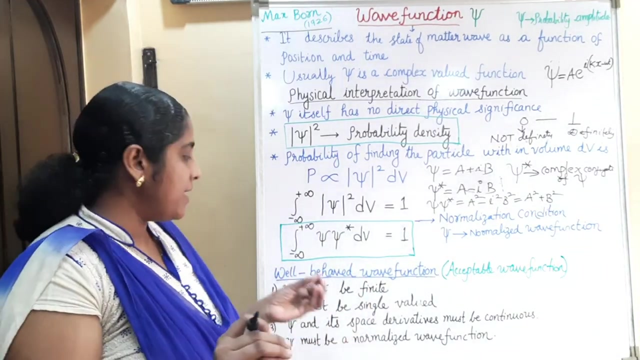 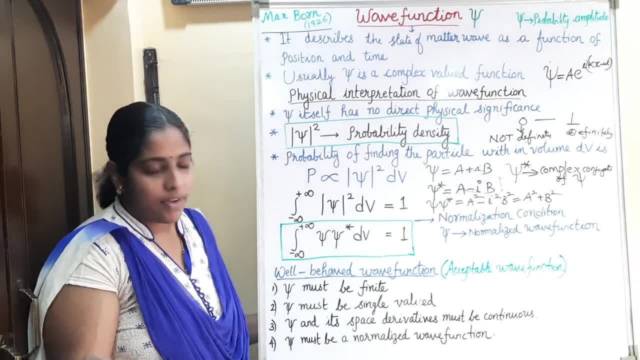 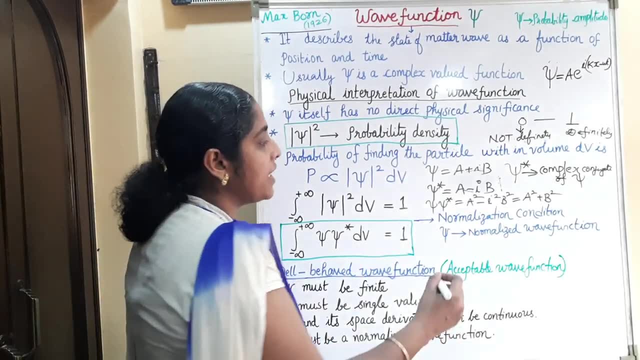 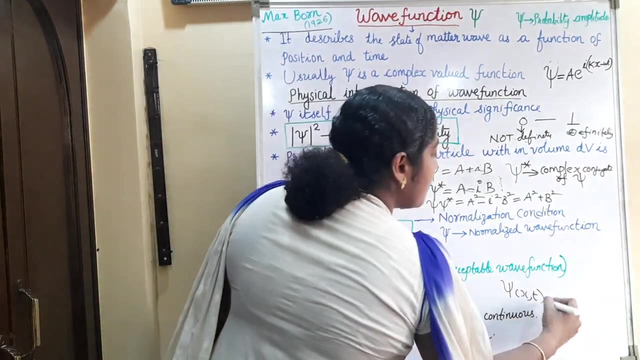 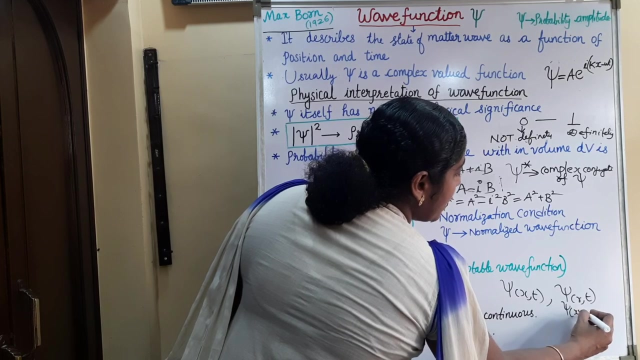 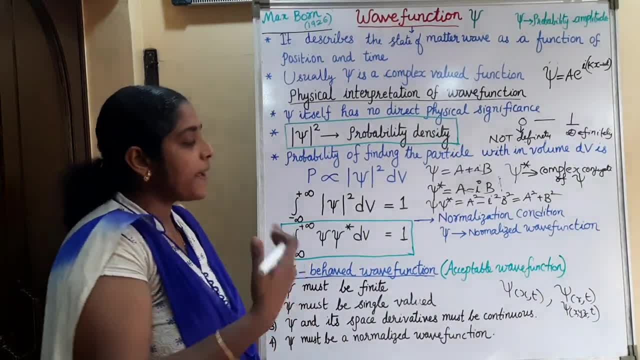 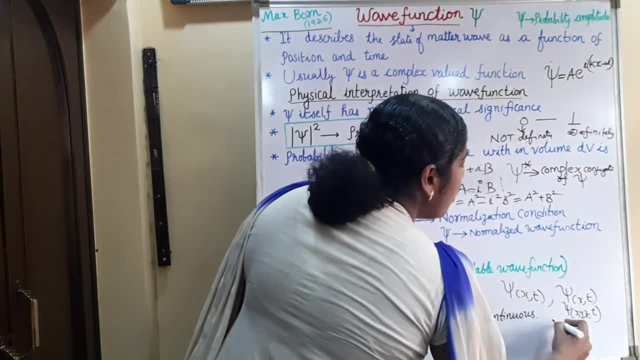 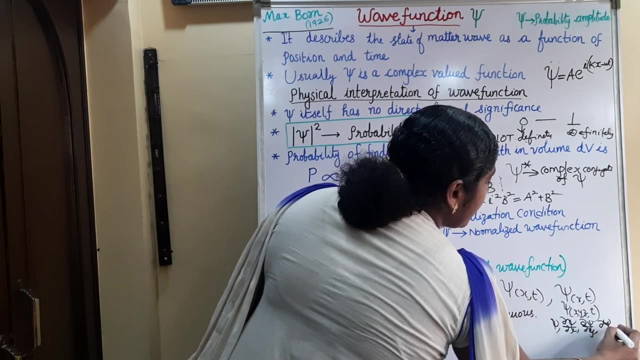 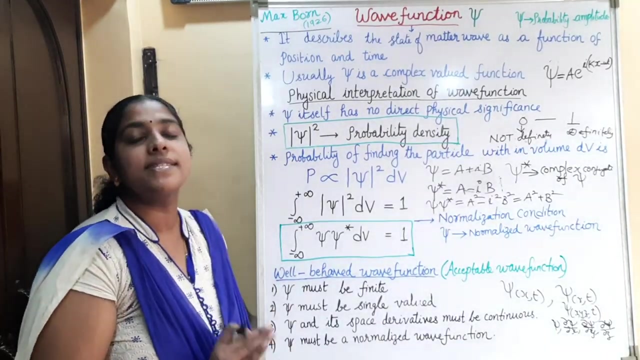 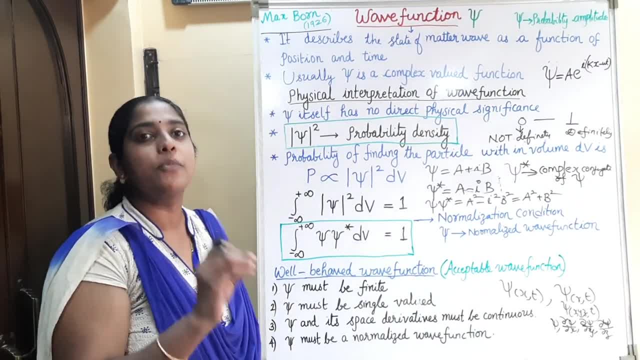 of the wave function. so this is the probability density of the wave function. so this is the probability density.